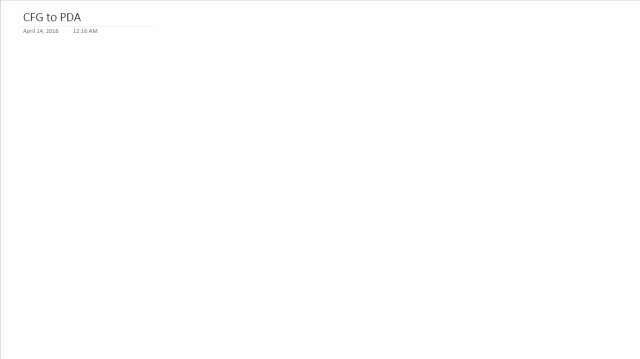 Hey guys, so this video should be pretty quick. Converting CFGs to PDAs is relatively simple. There's just a few rules to remember. So the first thing we need to do is we need to place the start variable on the stack. Number two, we have to account for all inputs on all. 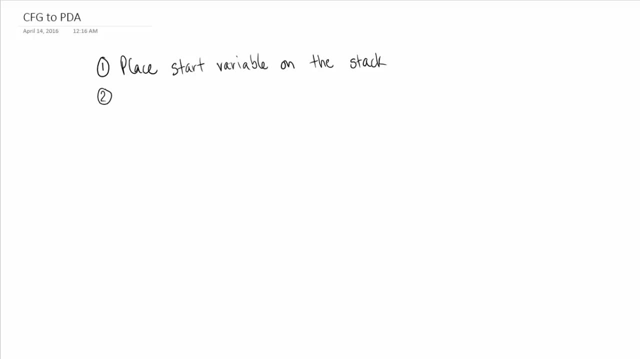 variables. So I'm going to be doing an example after I list these steps and you'll see what I mean. And for every terminal A, we want to pop it from the stack, essentially Okay. so I'll add a little example of number three here. You do this for every single terminal. 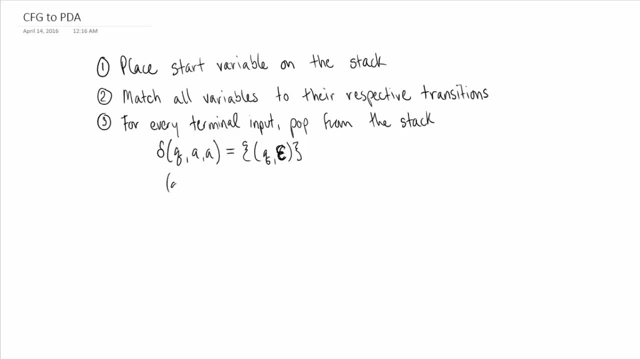 so if you have a terminal B, you do the same thing for B. So that would be like Q, B, B and then exact same thing. You're just popping from the stack. Now for this number three rule. if we end up with a grammar that contains something like this, we count epsilon as a. 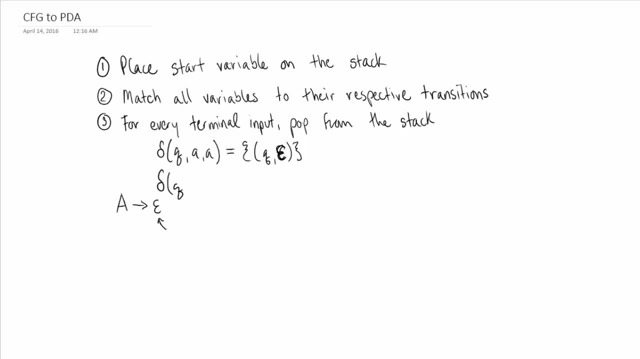 terminal. So we would end up with something like this: because an epsilon on a stack means popping from the stack, We're just going to use the empty stack symbol. So if we end up with an epsilon, we use the empty stack symbol here, Because we can't. 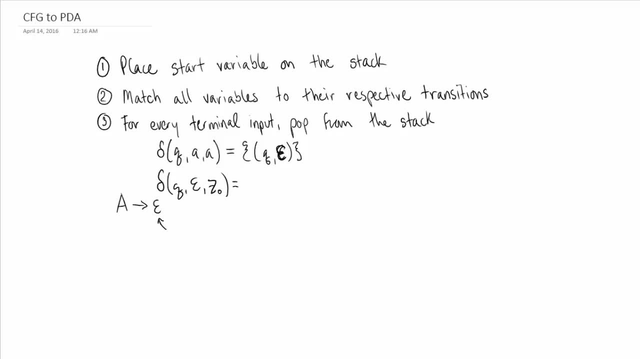 use epsilon on the stack. again that would just mean we're popping stuff, but that's not what we're doing on the left-hand side, but it's what we're doing on the right-hand side. So again, we're just treating it as a terminal. So let's try out a basic example. 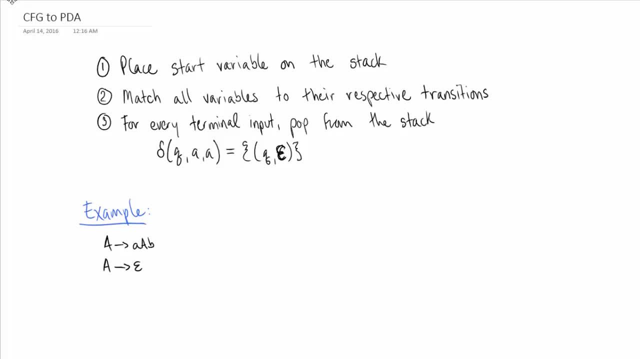 Okay, so for this one, our start variable is inevitably A, so we need to put A on our stack. so we have an epsilon input, we'll have an empty stack, and what we want to end up with is we want to end up back at Q. we're only ever going to have one state with these. 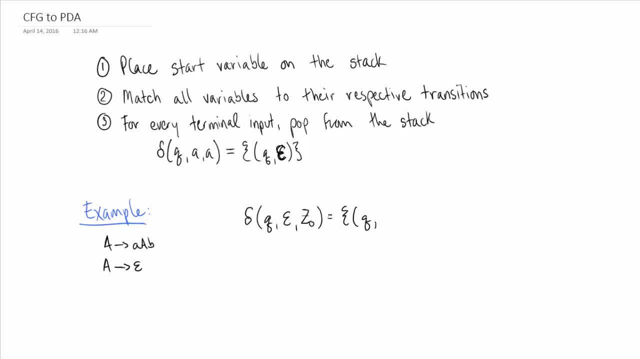 your PDA will always have one state and we're going to end up with with A on top of the stack. okay, now we're going to do step two. so on Q, we have an epsilon transition, but we have an A on the stack. we do this for all variables by the 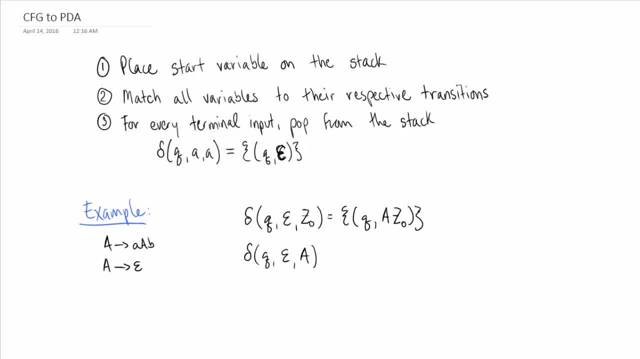 way. so if we had like little A, big A, big C then little B, then you would do this for big C as well. sound like a child: capital C and then Q, and we're matching it to its. 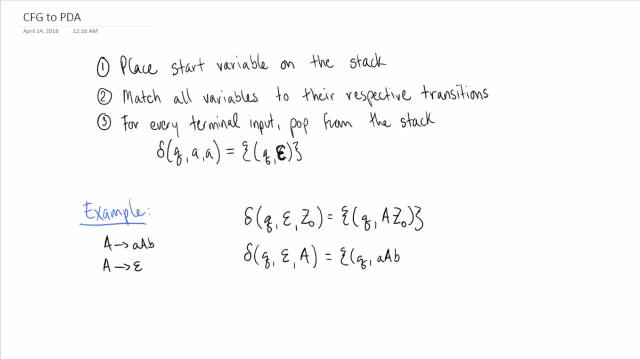 transition. so our stack ends up looking like that, and then we have another transition as well. Okay, so we're done. step two, and now on to step three. for each for every terminal input pop from the stack, right. so we only have three terminals, including epsilon. so 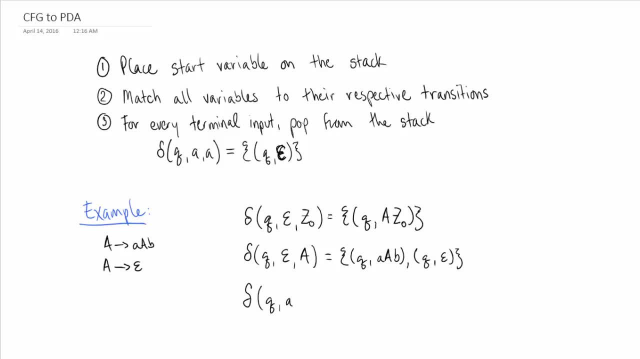 on Q. if we got an A and A is on the stack, then we're at Q again, Then pop and, last but not least, we account for the epsilon and again we do the empty stack symbol instead. Okay, so I'm going to move this here because now we're going to draw our PDA, so this is: